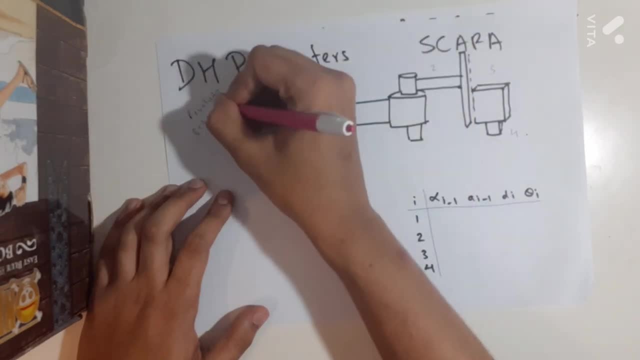 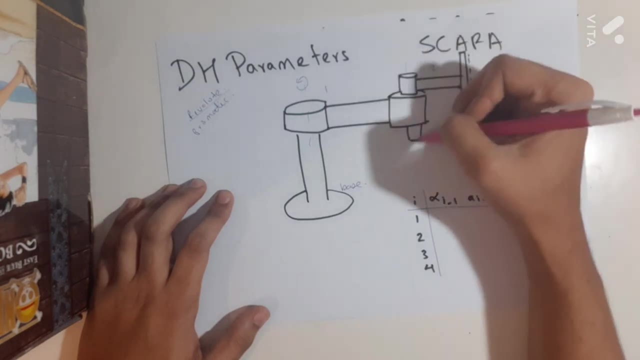 So what we are done is we approximately saving profits, and you can see here that these joints are not like hyvä knightไร joints, or are they prismatic joints? So first joint, def sized that it is a revolute joint, Then the second joint, over here as well, it is going to rotate. 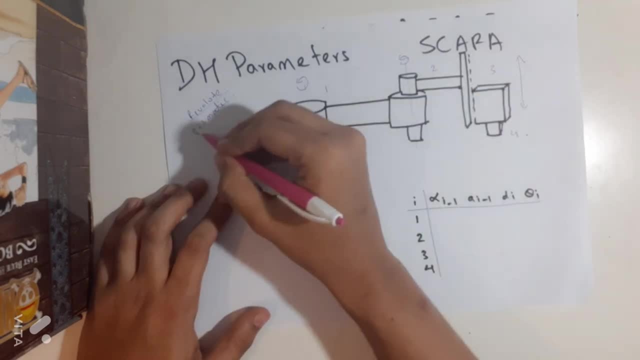 So on third axis, it's going to translate up and down. So this is a prismatic joint. On our fourth joint, it's basically going to rotate. Let's give this both the axis again. So this fourth joint goes behind the bridge and then the fourth one goes right up the bridge. 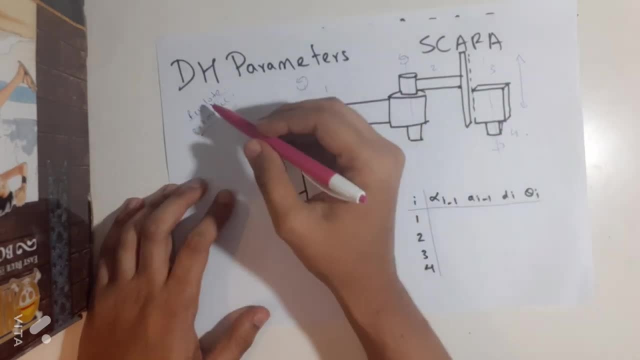 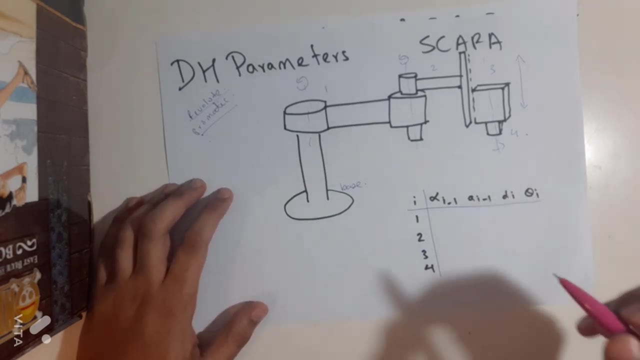 4th thing is going to rotate. So, as you can see, we have 1,, 2,, 3,, we have 3 revolute joints and we have 1 prismatic joint. So now we have got that figured out. Now, as you know, 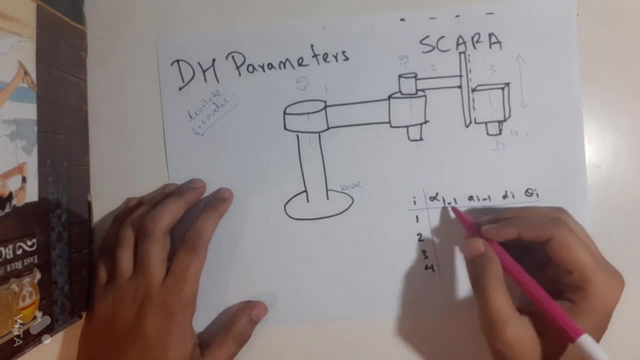 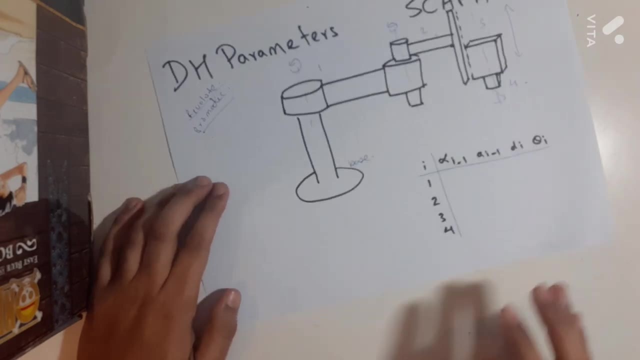 in DH we need to find 4 values. We need alpha a, d and theta. We will be understanding what these mean very quickly. So let's first see what is alpha? right, But before we go on to all of those things, let's first give the axis, First thing which you need to do. 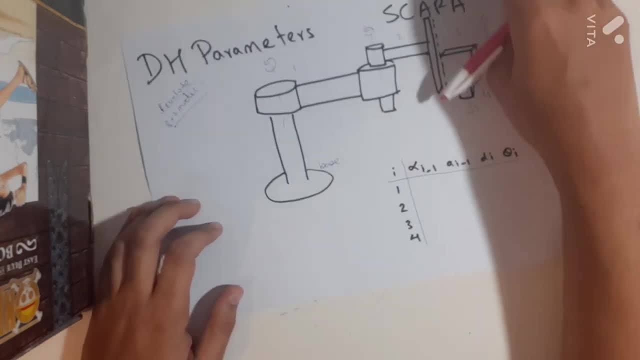 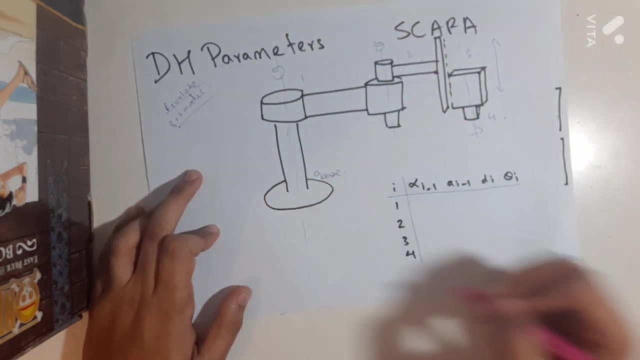 when you get a diagram like this is you need to give the proper axis. Over here, let's just call this 0. We can see that this is our revolute joint. We first assign the z axis about which the rotation is going to happen, About the base. it is this fixed joint. 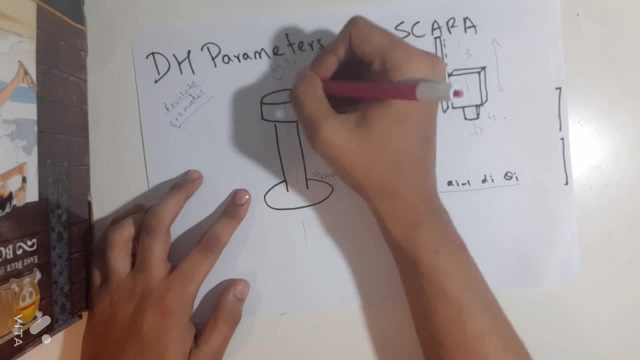 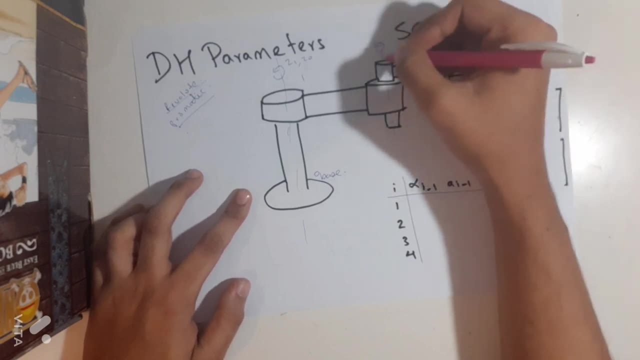 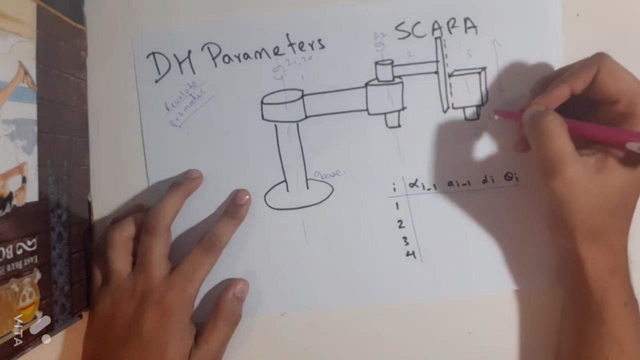 So let's just call this as z1 is for this, and we can also assign this Over here. we can see this is going to rotate on this joint, So we need to assign another axis over here. Let's call this z2.. Then for our 3rd and 4th link. So what's going? 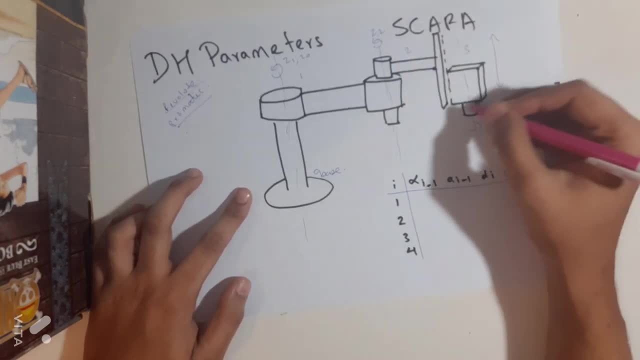 to happen is that our 3rd link is moving up and down and this is our rotational joint, So we can just give them an axis together and this axis is going to be our z3 and z4. Let's call it Right Now. what's going to happen is that. 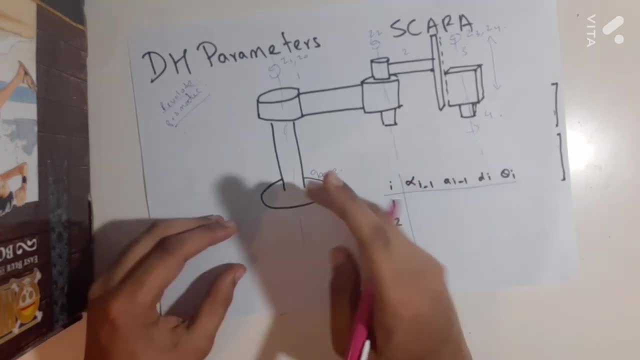 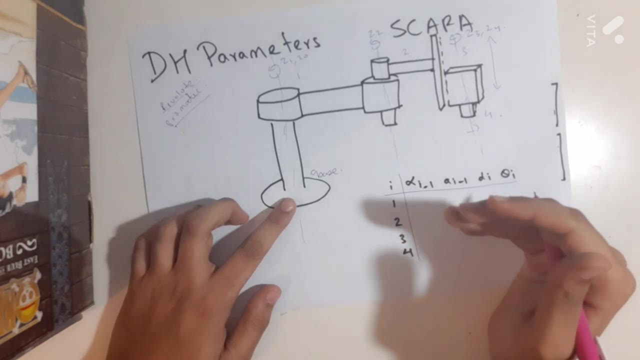 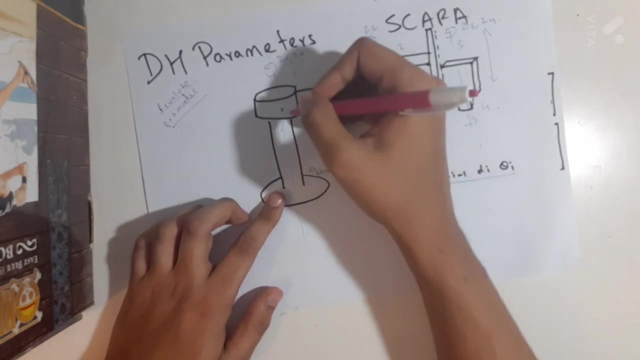 the next thing is that we are going to assign our first axis arbitrarily and the next axis will be dependent on the first, and so on. Right, So our first axis, again the fixed joint. Let's just mark it over here: On a fixed joint, you can put the axis over here. 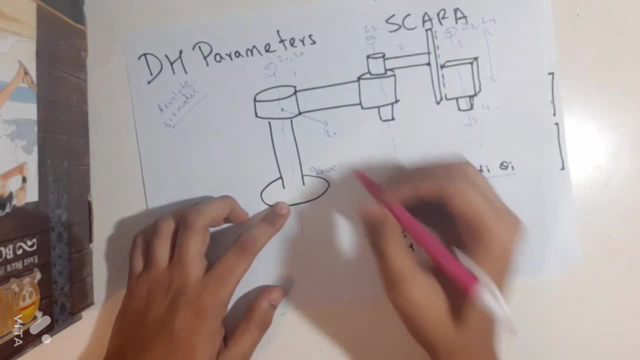 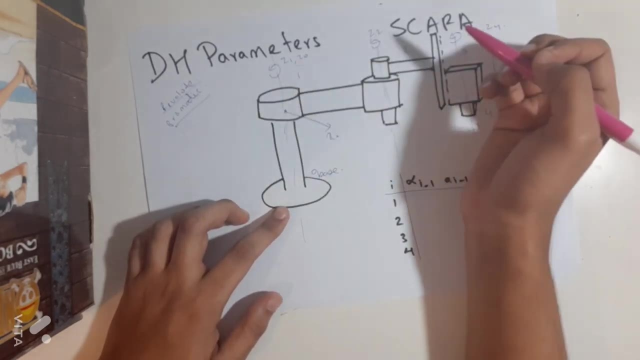 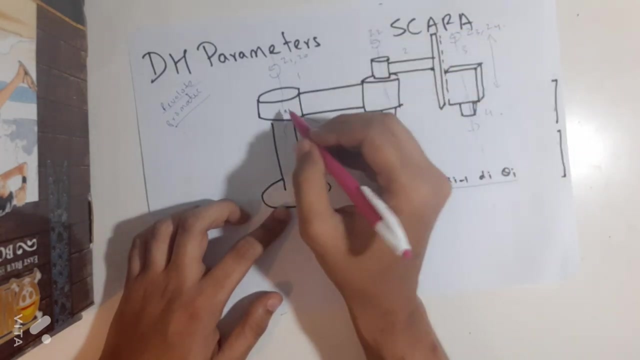 as well. So let's just call that. there is an x0 over here. This is the x axis for the base. Now what we need to assign is our x1.. So our x1 is basically perpendicular to our z1 and our z2 axis. So basically it's going. 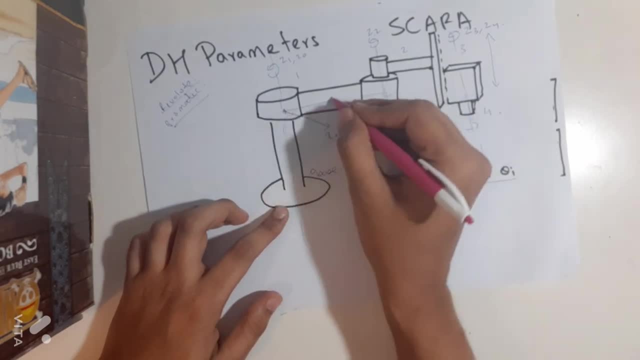 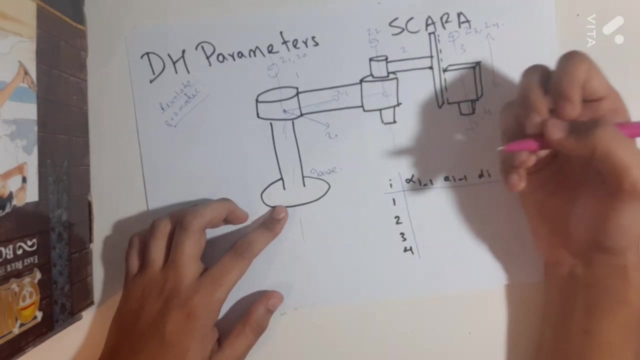 to be perpendicular to these both. So this will be our x1.. So, just to relate to the dh, let's just show you that the angle between xi and xi-1 along the z axis is basically your theta. So this is actually going to be our theta1.. You will see that later. We. 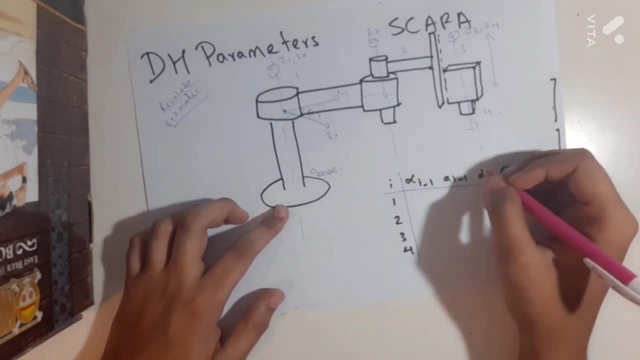 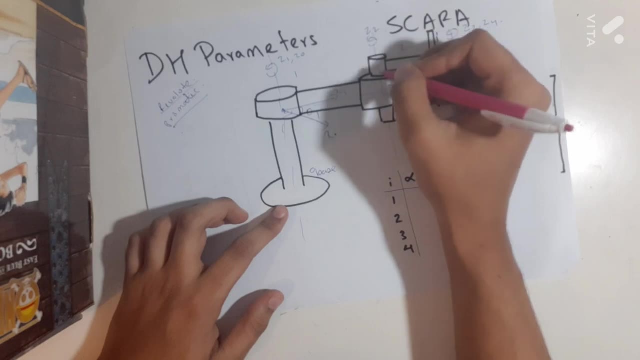 will fill up this table Right. So that is your x1.. Now this joint right we need for our x2, what we are going to go is we are going to go joint by joint. So our z2 and our z3.. This is our z3.. So 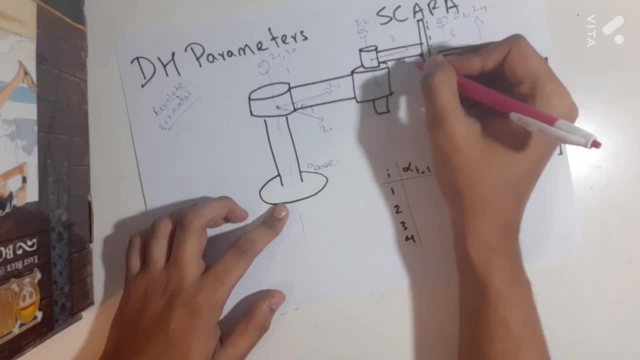 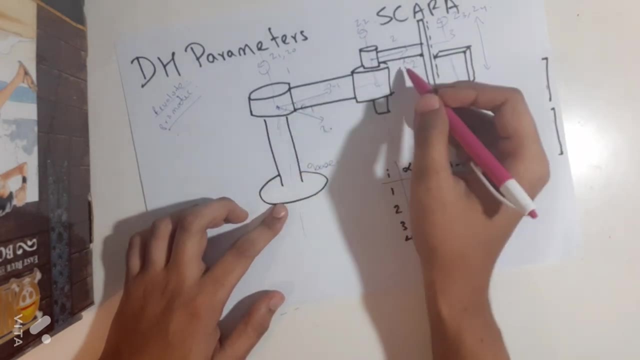 perpendicular to both of these, we are going to get our x2.. So our x2 is over here. Now you might think that x1 and x2 are in the same line, but that is not necessarily true. Like, let's say, both of my arms are that joint? 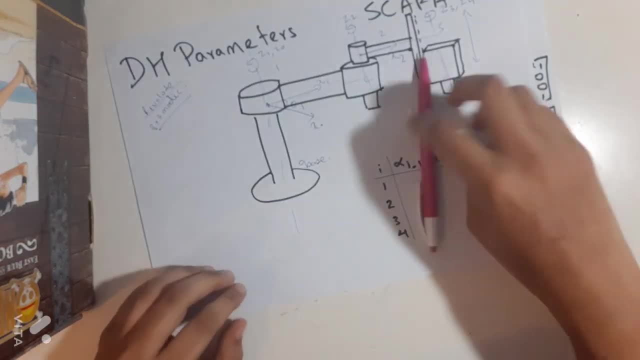 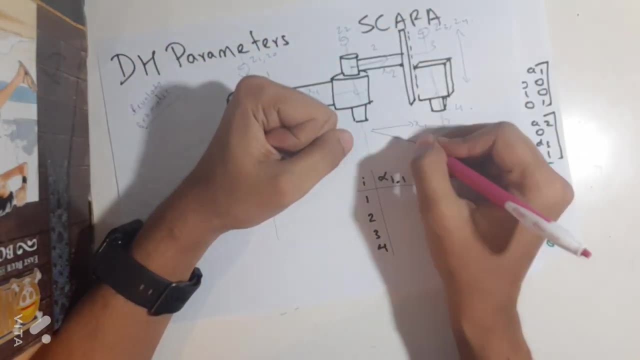 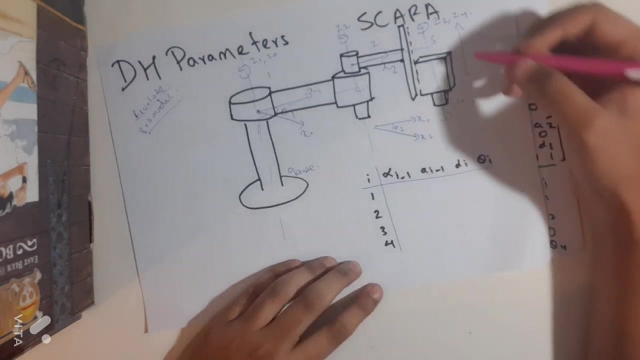 Our x2 axis can rotate, So there can be an angle form between x2 and x3.. So our, let's say, x1 is going like this: Our x2 can basically rotate like this and you can have an angle between x1 and x2.. Right, So that is basically going to be your theta2.. Our x2 is over here. 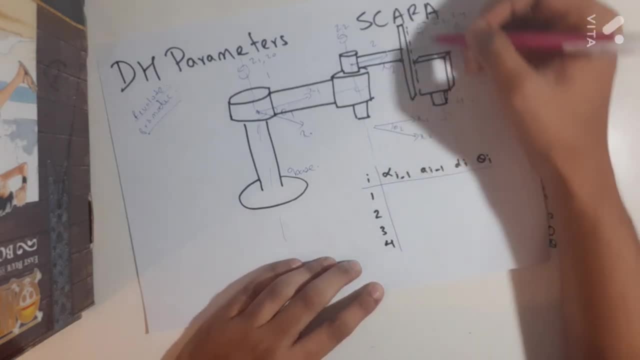 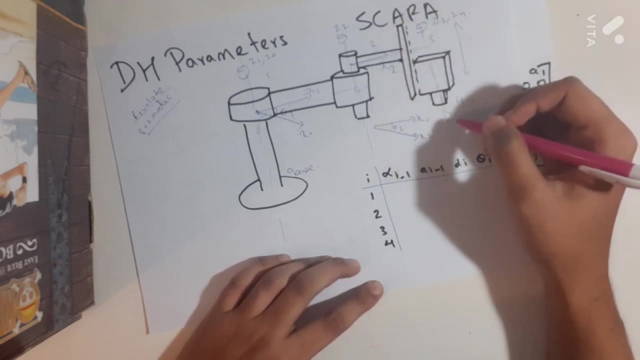 It's going to extend like this: Now our third link, Our third link. what it's doing is it's not exactly rotating, It's just translating up and down. So what we are going to do is we are going to assign our x3 over here, Right And because, 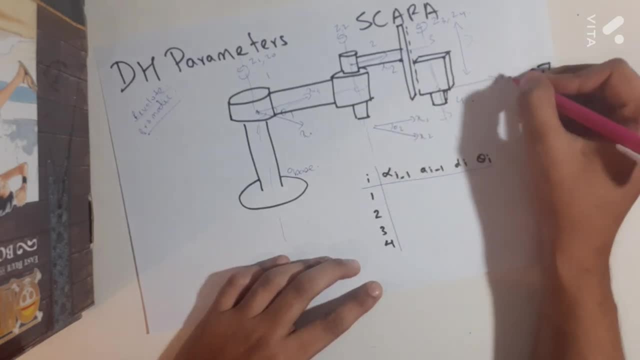 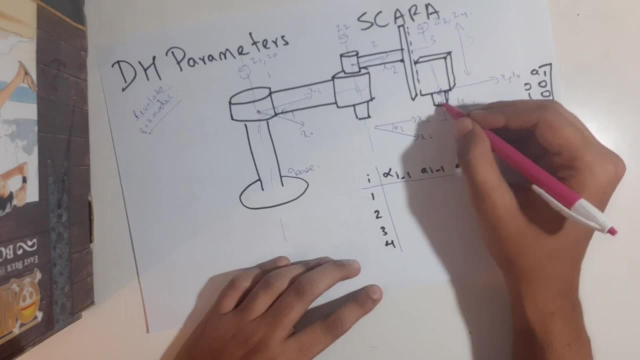 our x3 and our fourth link are at the same point. we are also going to assign our x4 over here. It's basically we are doing it over here, but just remember that x4 we are assigning for this joint and our x3 is being assigned for this link. So like x4 is for this link, 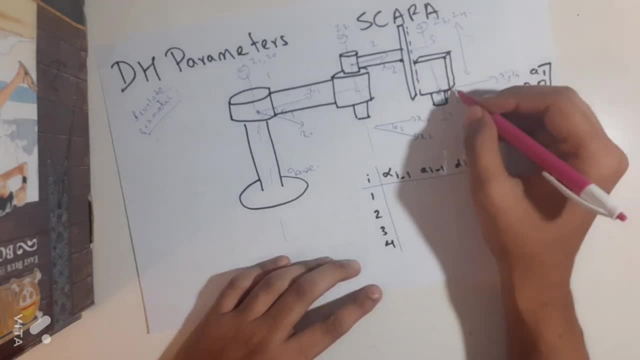 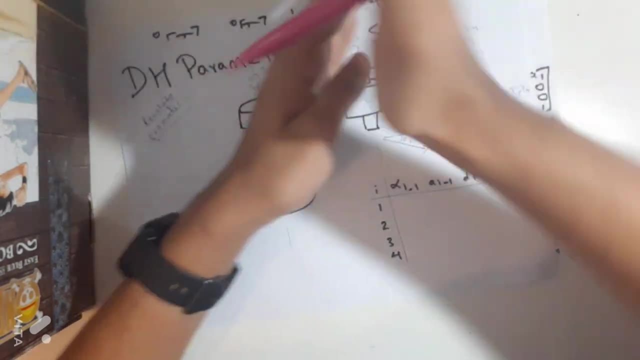 x3 is for this link. We are assigning it together, but you can think of it as two lines over here. Now you know that our x4 can rotate. So basically our x4 and x3, let's say they are. 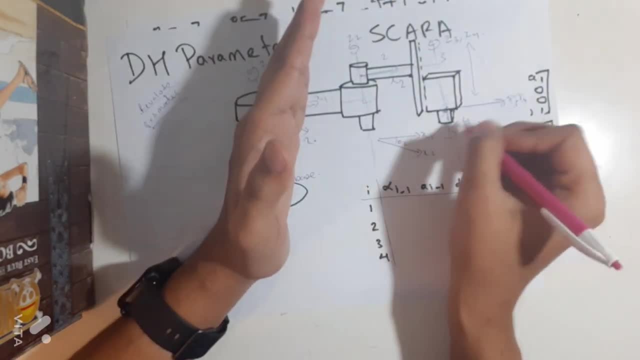 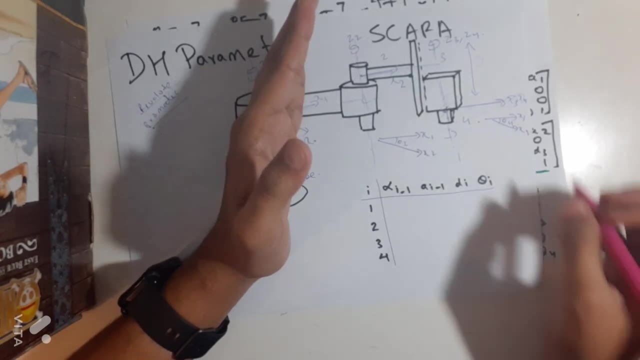 on the same line, but our x4 can basically rotate out because this is a revolute joint, So there can be an angle form between x3 and x4 as well. That is actually going to be our theta4.. So, as you can see, we have just marked our axis for the entire bot and 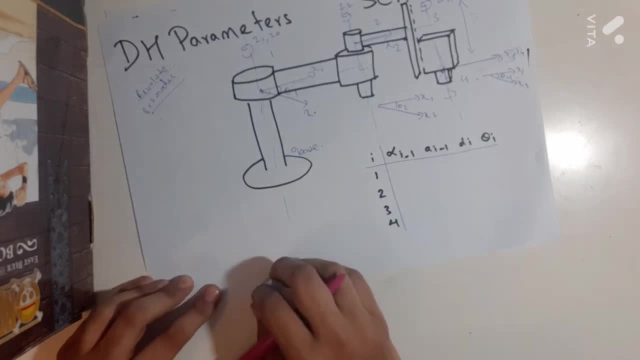 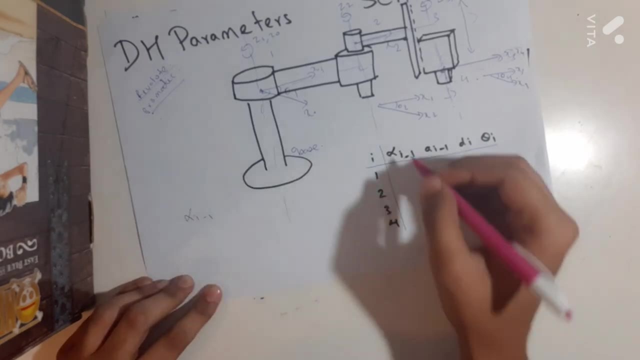 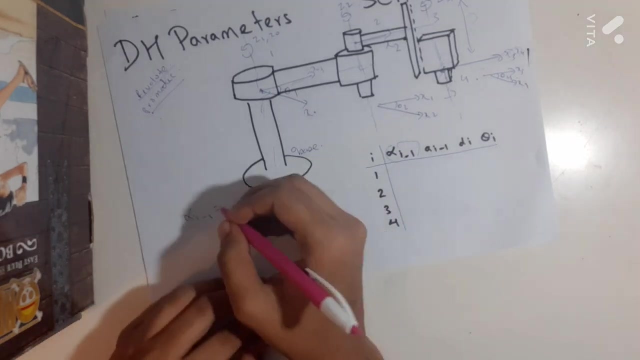 now let's fill up this table. Filling up this table is actually quite easy once you remember the equations. So what is our alpha? Basically our alpha. don't think of it in turns of formaben, try to think of it like physically. So alpha is basically the angle between our 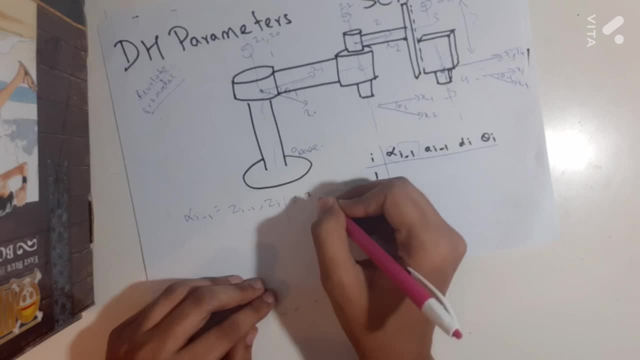 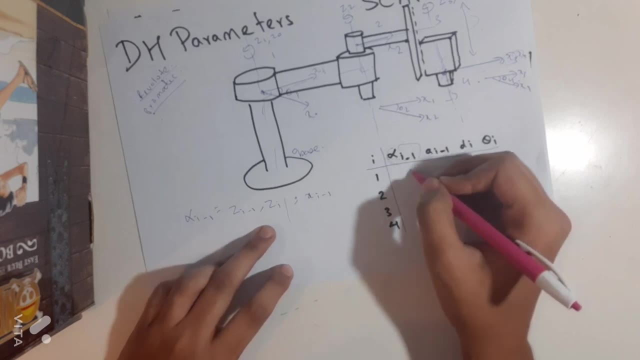 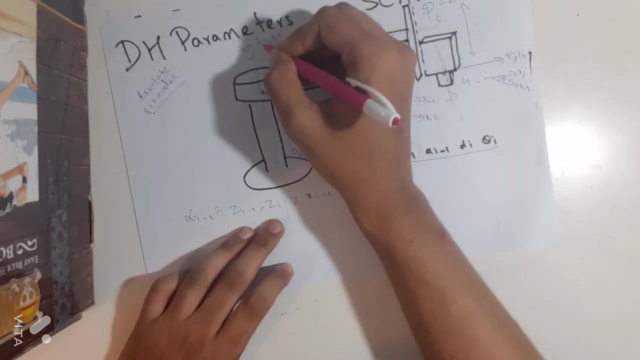 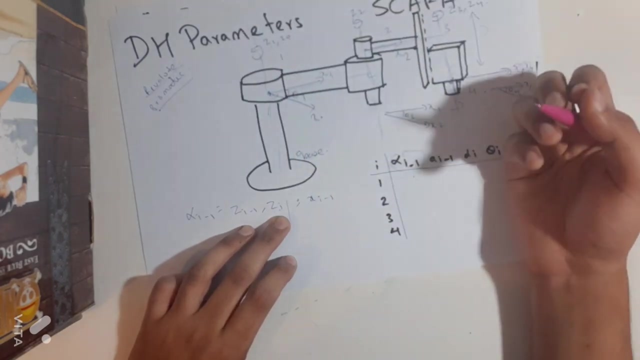 zi, and it is along our x-axis. So let us say we are going for alpha0, right? Our alpha 0 is actually the our z0 and z1 axis, because z0 and z1 along our x0. Now you know that our z1 and z0 is. 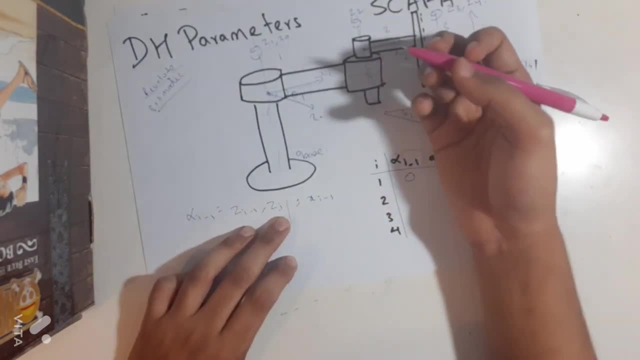 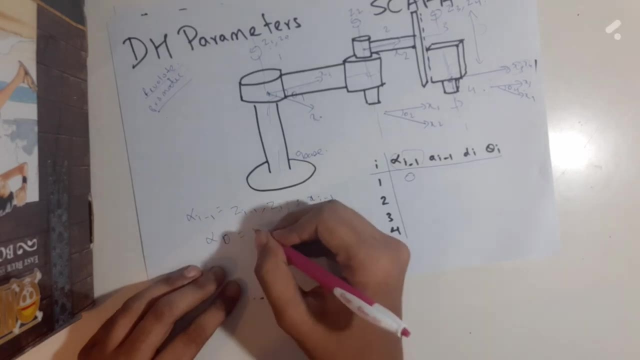 the same axis, so we are going to give it 0.. Now let's go for the next one. So our alpha 1, 0 was basically z0 and z1, the angle between them. Our alpha 1 is going to be the angle. 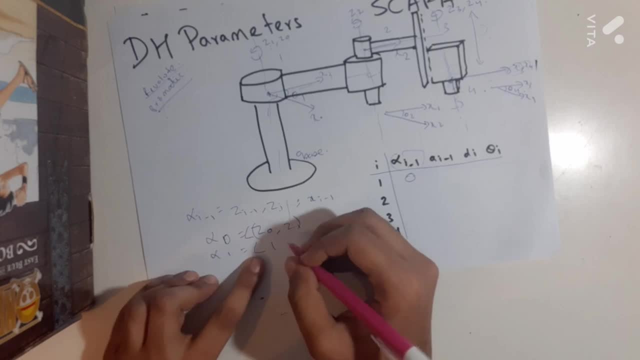 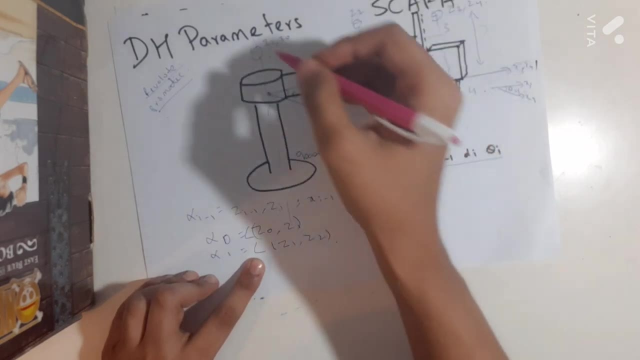 between our alpha. 1 is going to be the angle between our z1 and z2.. So, as we can see, this is our z1 and z2, they are parallel, So the angle between them is again going to be 0.. 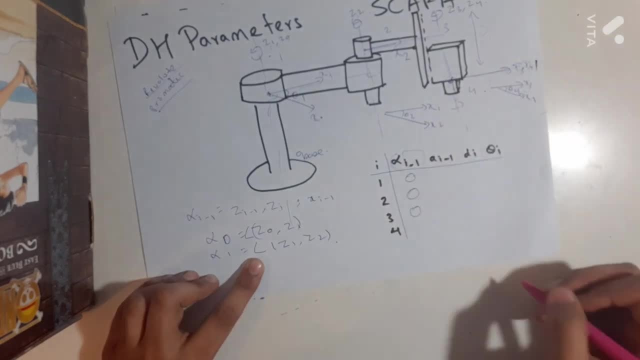 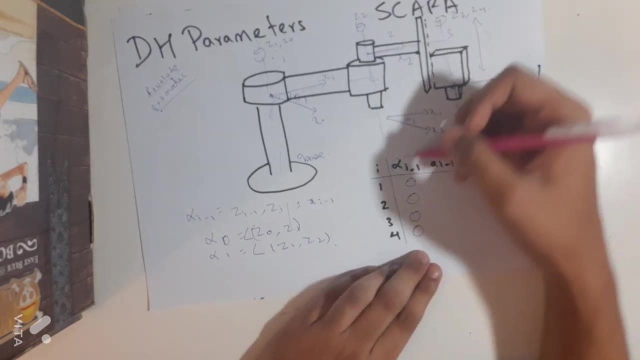 As you can see, the same is going to happen for z2 and z3.. The angle is going to be 0 and our z3 and z4 is the same axis. So in scalar robot your alpha i-1 is going to be: 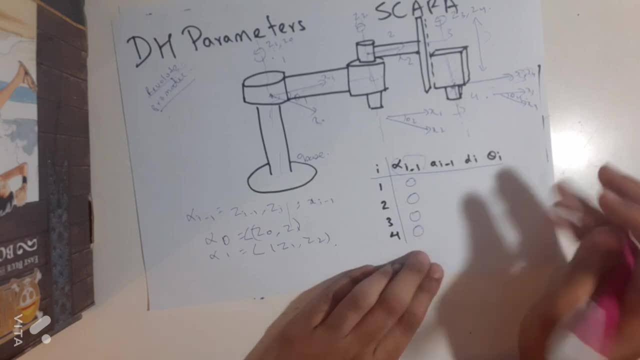 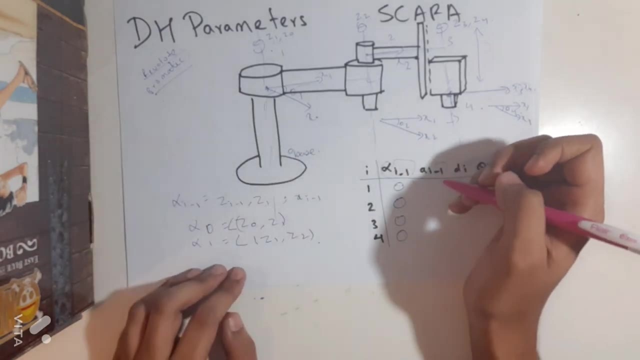 0 for all. Okay, Okay, Okay, Okay, Okay, between your z axis. now let's go for the next parameter. what is a minus 1 a is basically your length, right? so your link length is the length between your axis. so, like over here, our z1 and. 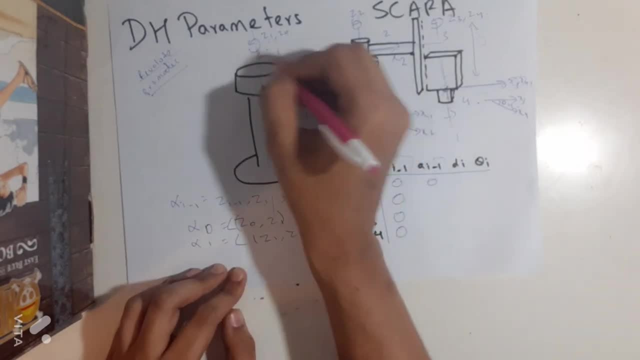 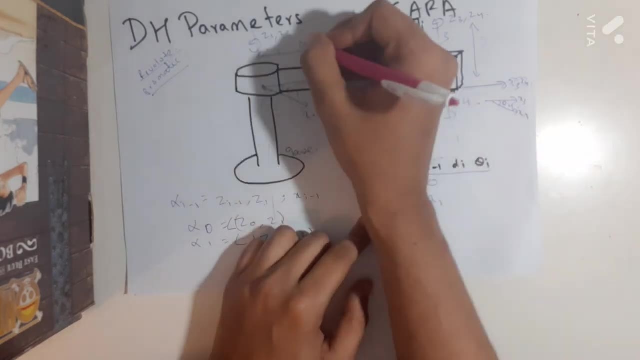 z2 is same, so it's going to be 0. this is going to be the link. length for i is equal to 2, basically a1. so we are going to give this a1. this is your a1. then for our i3, that means a2. the the distance. 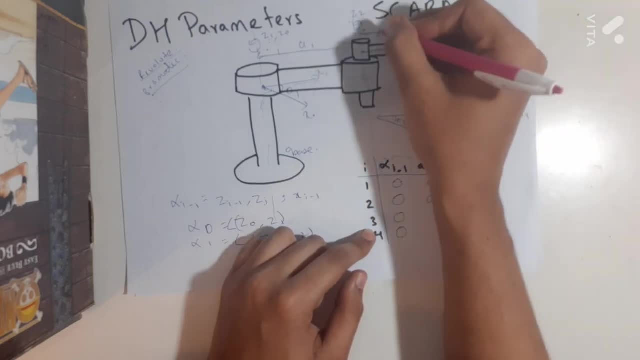 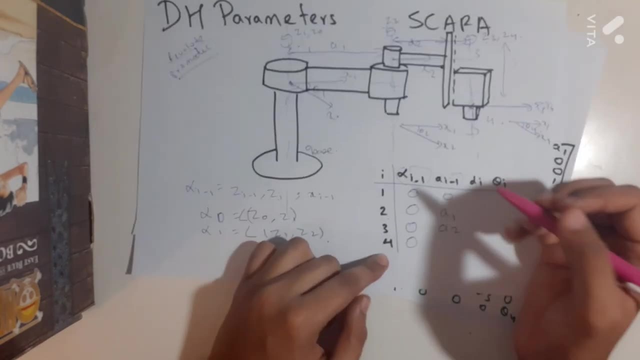 between z2 and z3 is basically going to be your a2, so you're going to give your a2. our z3 and z4 are the same axis, so again we can't have any distance between them, so it's going to become 0. 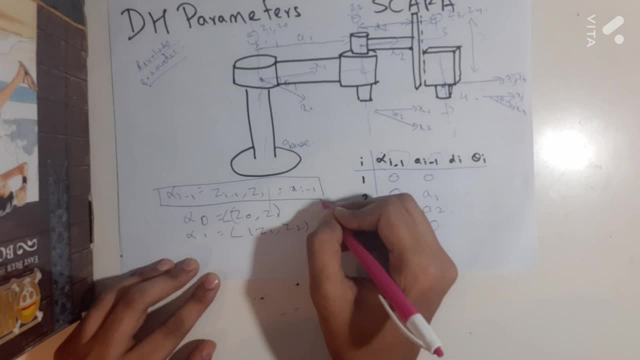 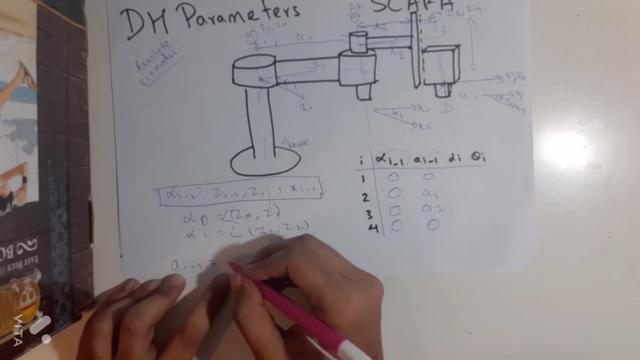 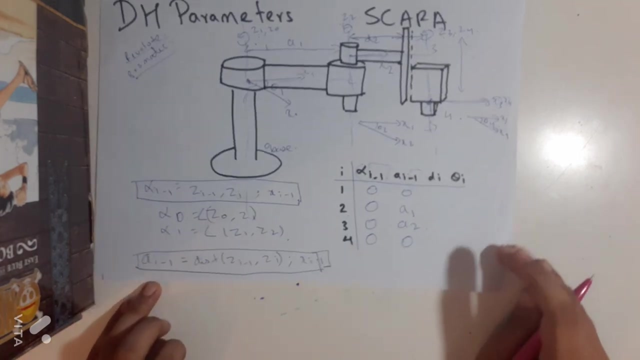 so, just the way alpha had this formula, a has this formula in the sense. so the link length is basically the distance between zi-1 and zi along xi-1.. So that is your link length formula. So we have filled out that now. Now let's move forward. What? 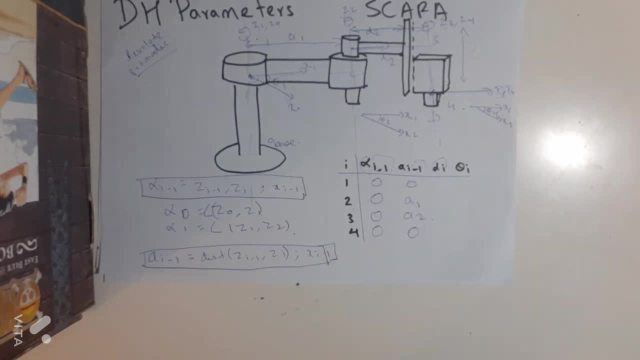 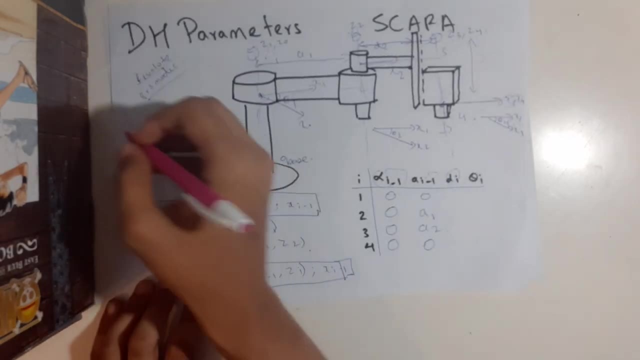 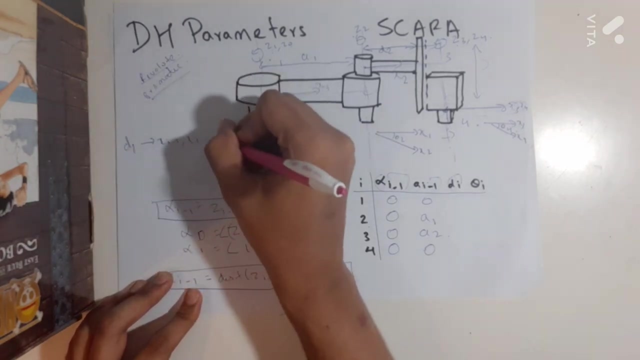 is our d. Our d is basically our offset. So d is the offset between your x axis and it is along the z direction. So you can write d as this. di is basically the offset between your xi-1 and xi along the zi axis. So as you can see over here, it is in the same plane. 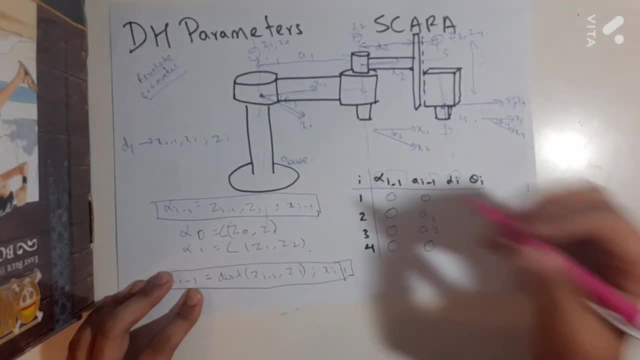 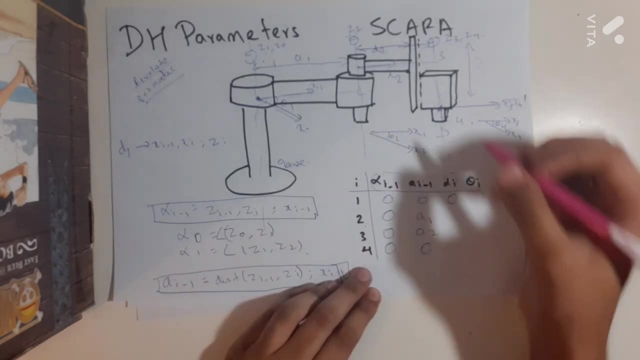 You can see that we are drawing xi-1 and x0 from the same point right. It's in the same plane, So there is no offset between them. So your di is going to become 0 for 1. Over. 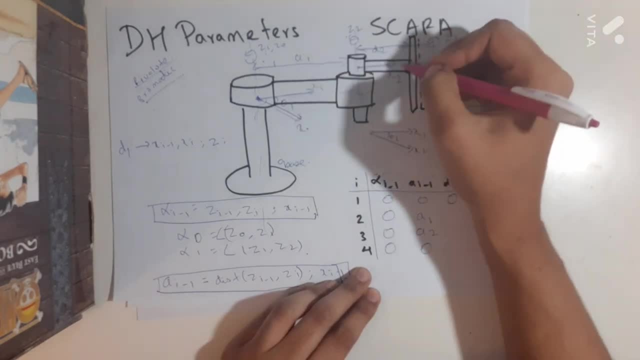 here you can see that actually our x1 and x2 are the same. So you can see that our x1 and x2 are the same. So you can see that actually our x1 and x2 are the same, So you. 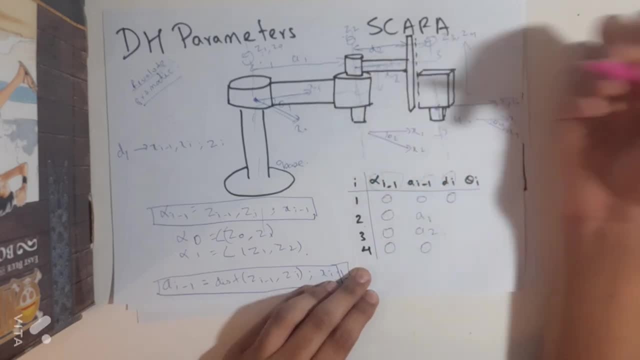 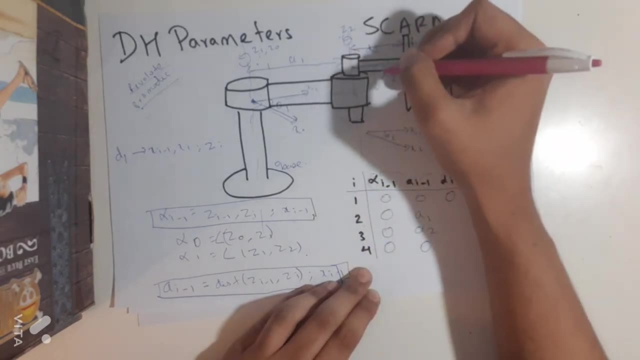 same plane. we are drawing this, but this is very minimal distance, as you can see. like in most color robots, this will be side by side. this is in the same joint. i've just drawn it like this. so actually the distance between our x2 is over here and x1 is over here. we draw it in the same 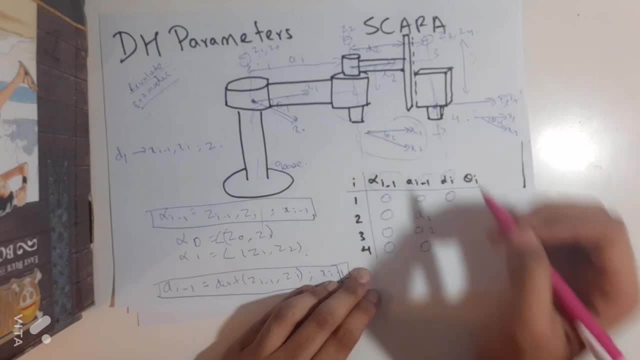 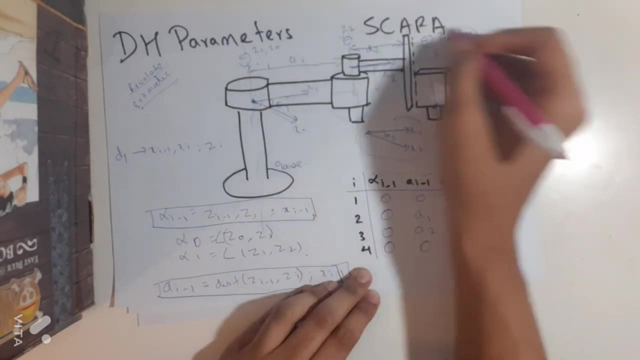 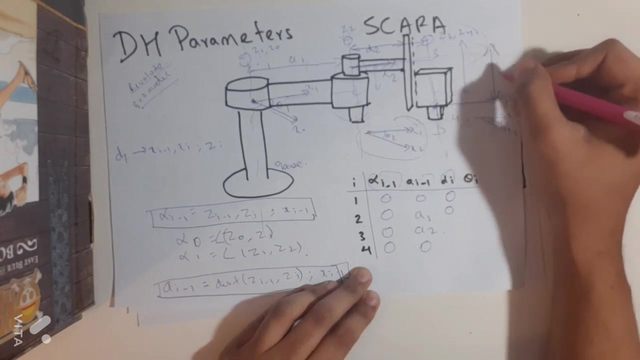 plane. so because it is in the same plane, starting from the same point, then the offset is again zero. you can see our x2 is going like this, like in this plane, this entire plane, and our x3 is over here. so you can see that there is a distance between our x2 plane and our x3 plane. 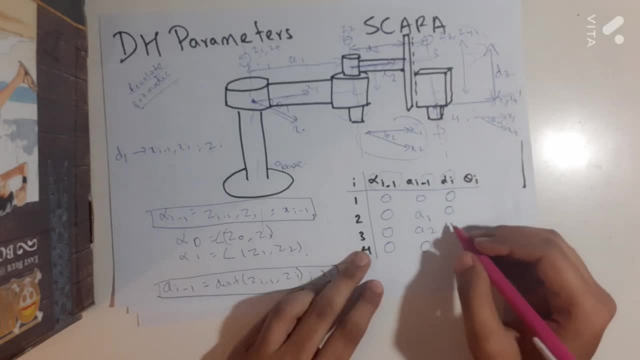 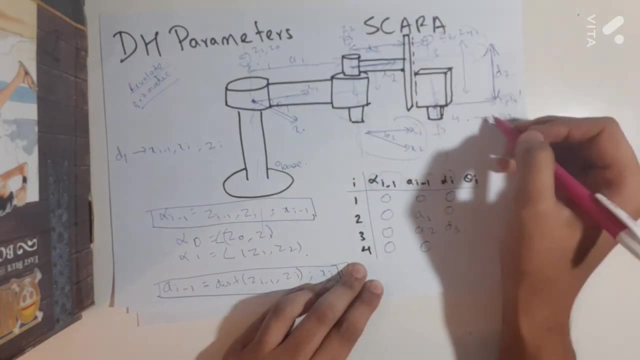 that is basically our offset over here. so for our i is equal to 3. it's going to become d3. this distance basically, as you can see, the planes have changed between your x axis along the z axis. this is the z-axis along the z-axis, the distance between our x2 and x3, that is d3. so that is our. 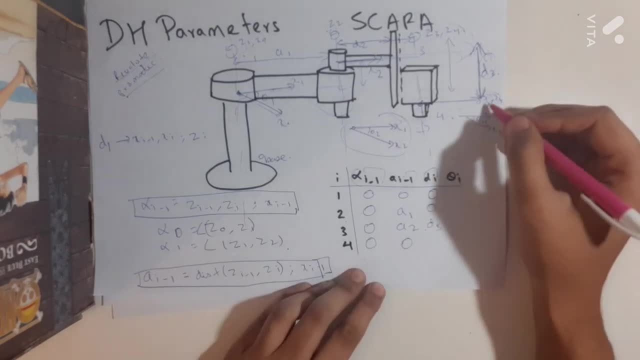 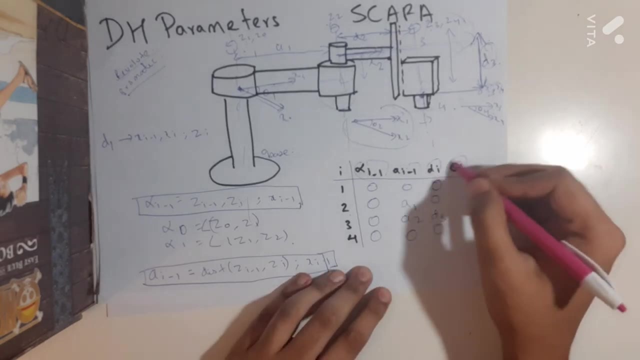 offset over here. so di is equal to d3 and our x3 and x4 again originate from the same same point, same plane, basically. so our offset is going to be 0 again. Now, what is theta? I think I have already shown you theta. Theta is the angle between your x axis and it is 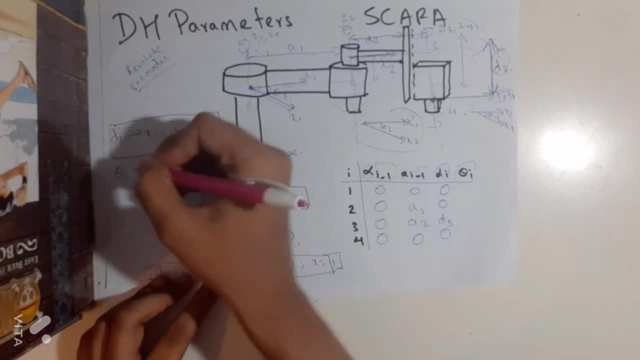 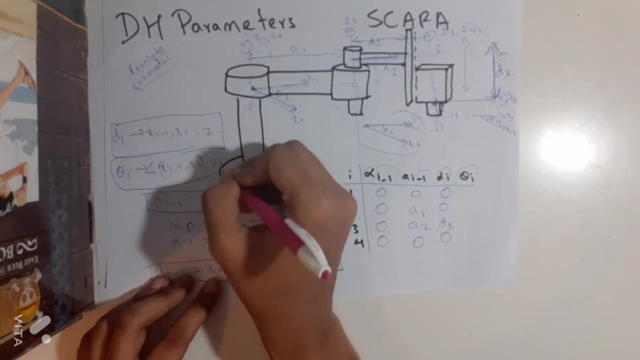 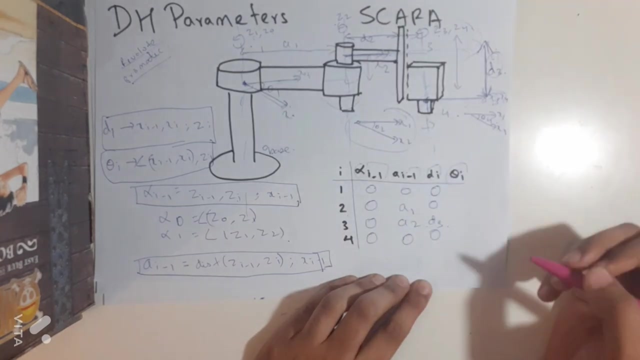 along the z direction. So you can write theta: i is basically the angle along your xi-1 and xi and it is along your zi direction. So that is like the formula for it, if you want to remember it. And let's just mark theta. so theta-1 we have already marked for i is equal. 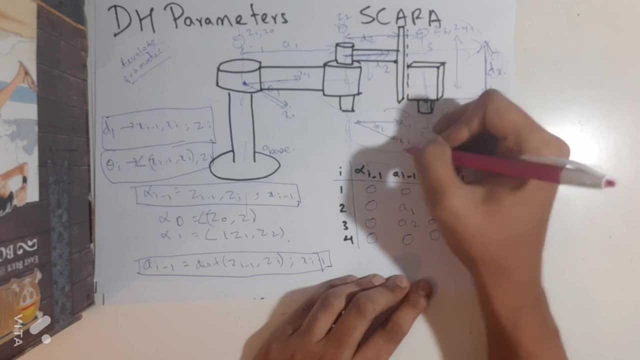 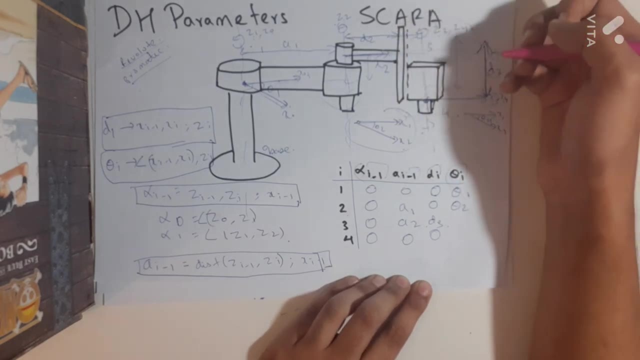 to 1 is theta-1.. Theta-2 also. we have seen the angle between x1 and x2, so that's theta-2.. As you can see, this is a prismatic joint Right In our prismatic joint. one more thing. 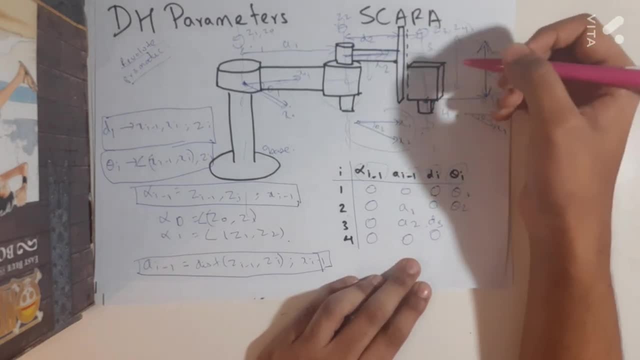 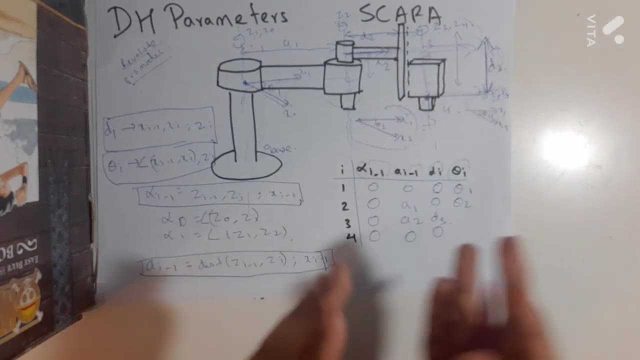 which you will see, is that there is no angle formed between the x axis, like this x2 over here, like our x2 over here and over here. They are going to be the same angle, So like they don't have any angle difference between them, The only difference is the offset. 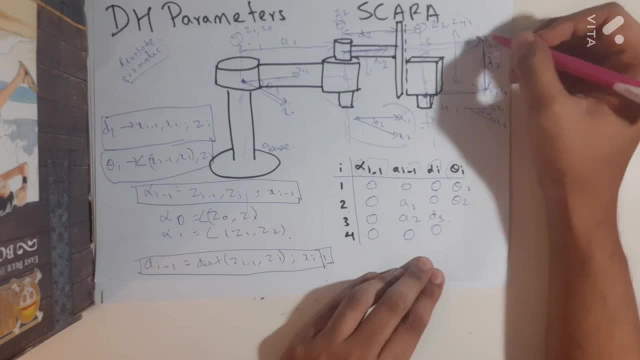 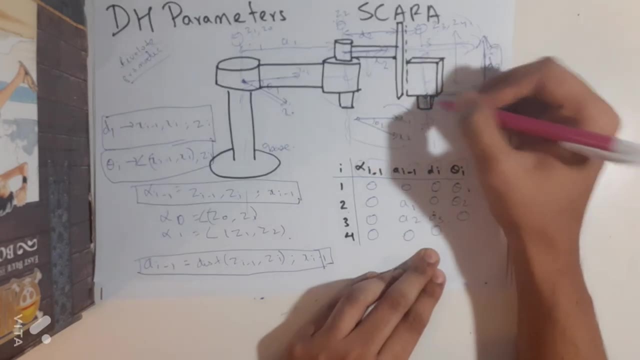 which is our d3. So actually a no angle is formed between x2 and x3. So it is going to become 0. And we have seen that at this joint. this is for the revolute. x4 and x3 is basically. 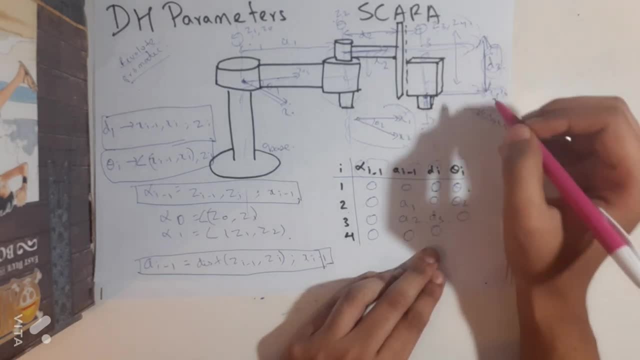 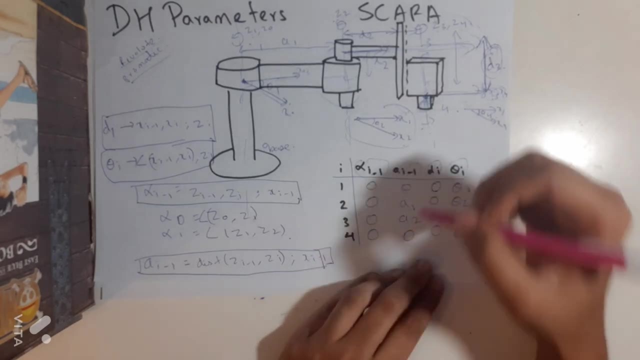 for this link. So what is going to happen is that there is an angle going to be formed between them when this joint is basically going to rotate, So that is going to become your theta-4.. So now you have seen how you can basically 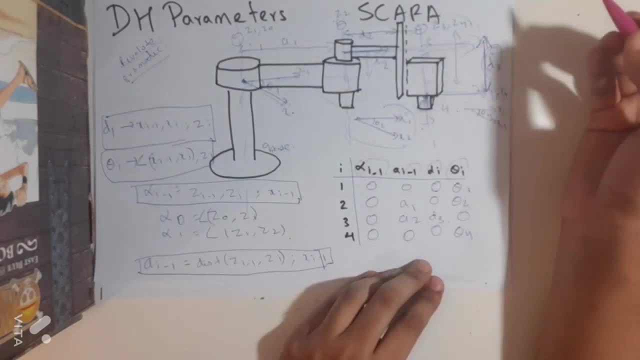 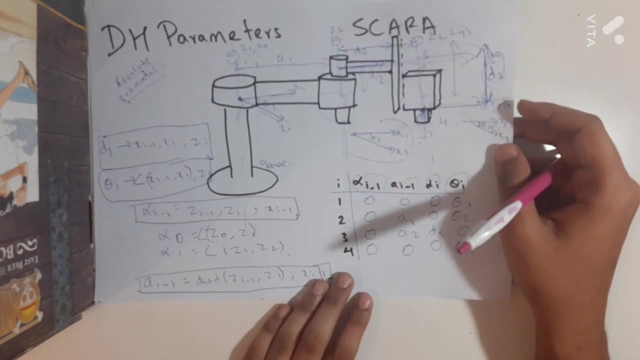 give those angles, Those values to the entire diagram and how you can analyze it. Right, But what was the entire point of this? We are trying to find the x, y, z coordinates based on our dh values. So let's go forward. What we are going to do from this is we are going to make a transformation. 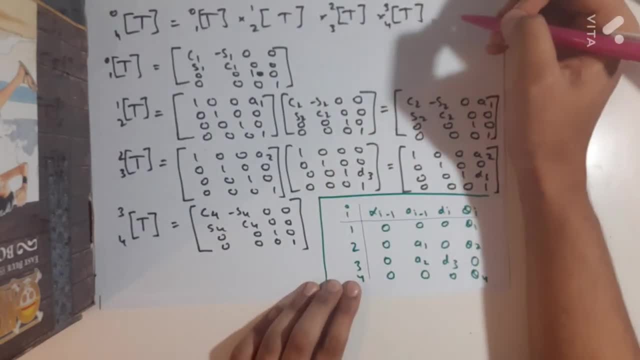 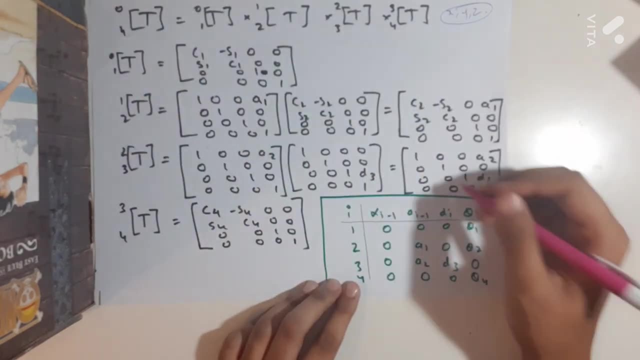 matrix. We want a transformation matrix which will give us the value of x, y and z, Right. So basically, we want to analyze all joints from 0 to 4.. But now that is too hard. So what you can do is you can go back. 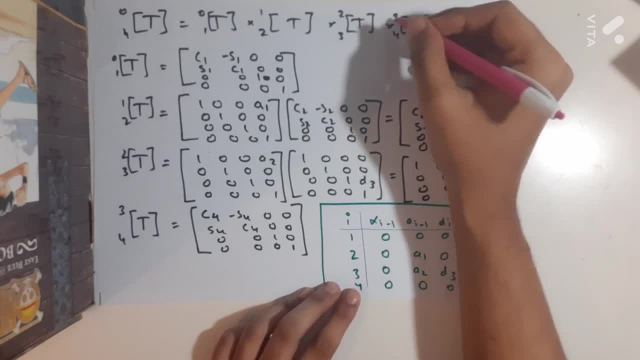 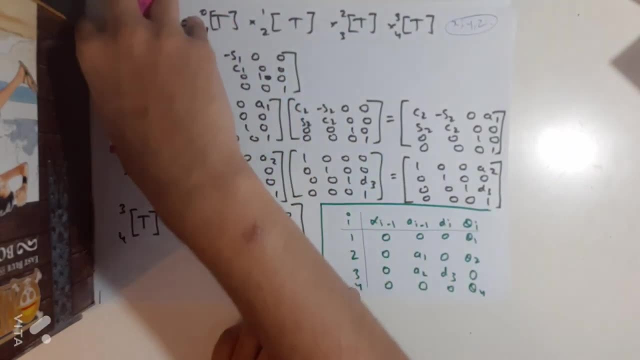 joint by joint. So you can basically see your transformation from fourth joint to third joint, from third to second, second to first and first to zero And you can multiply all of those to get that final transformation Alright. One thing which always helps while you are writing the transformation matrix is having 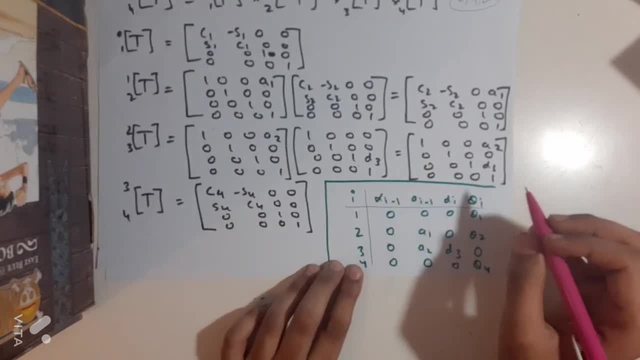 this table handy. So you will see that we, how do we write this? transformation matrices, matrices. let's just take a very easy look into it. you basically group these two and these two together. these are basically for your x and these are for your z. all right, and according to them, 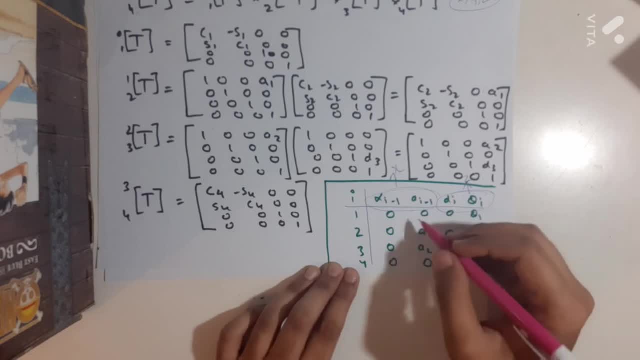 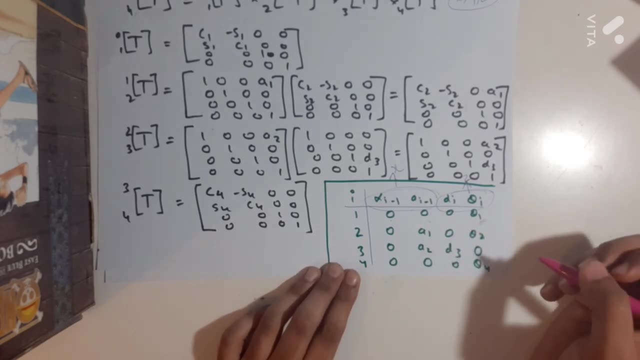 you are going to be writing your transformation matrices, so your first- you can see this- is 0: 0. so we are only going to actually need one transformation matrix. now, here there is a rotation, there is an angle, so for that we have a set formula in transformation matrices. you have. 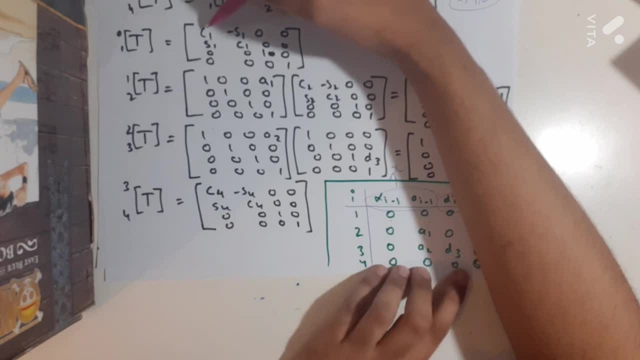 learned you must. you can go ahead and learn why it is like this. so you are going to have your c. whatever is your theta value over here it's theta 1, so it's your cos: theta 1 minus sine theta 1: 0, 0. 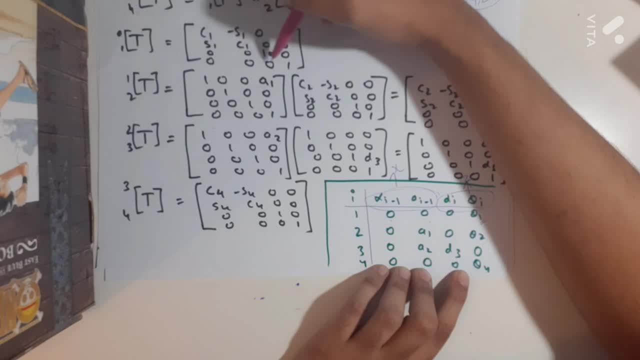 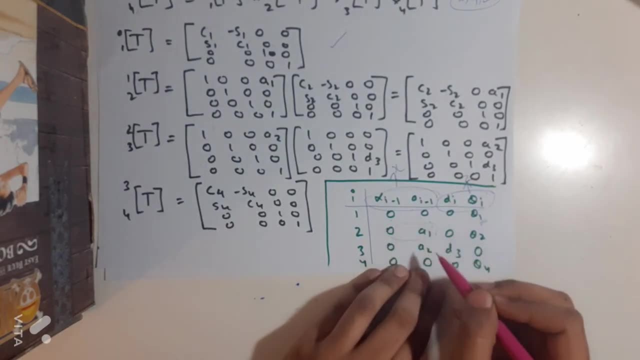 sine theta 1 cos theta 1 0 0 0 0. 1 0 0 0 1. all right, so that is our first transformation matrix done now in your second transformation matrix you can see that there is translation over here. 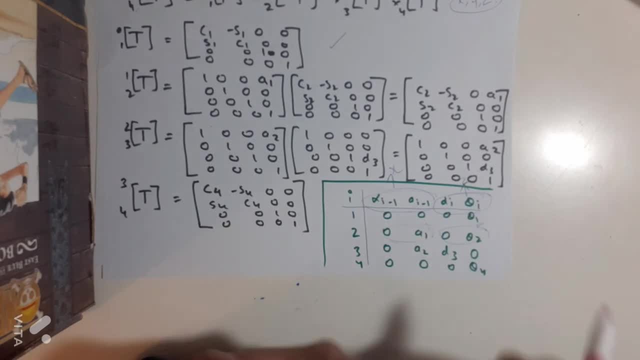 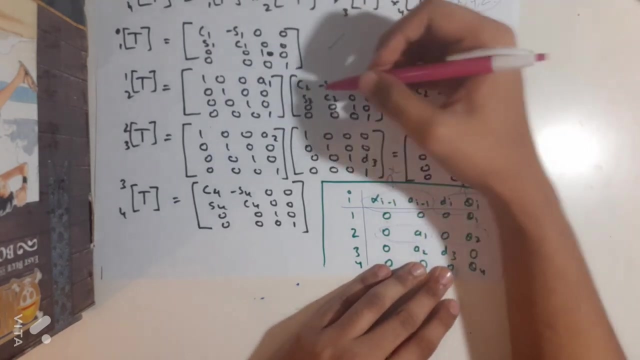 and then there is rotation. you can write both of these together because there is no rotation in the other one and there is no translation over here. so it is possible to write them together. but just showing you for the process, what we have done is first we have done the translation over here along a1 and then we have rotated it by theta 2. 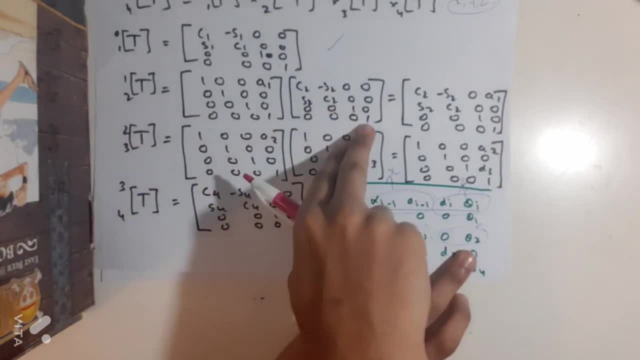 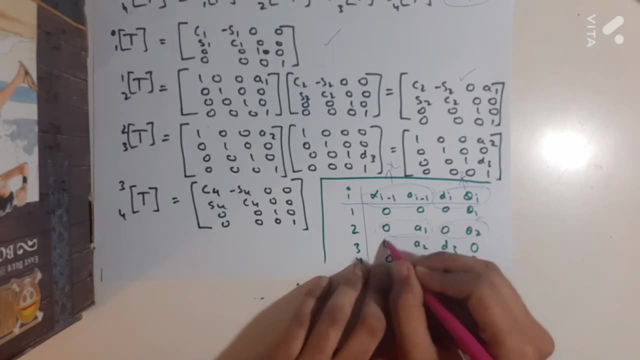 and we have multiplied those two translation and rotation transformations together to have our second transformation matrix in our t 2 to 3. you will see again, we have one translation and we have another translation again. so, as you can see, we have again. we have written it for translation. 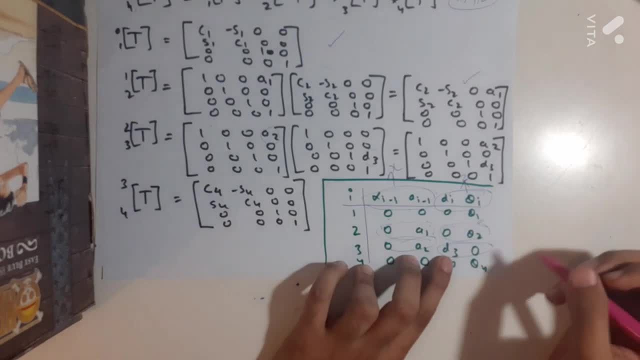 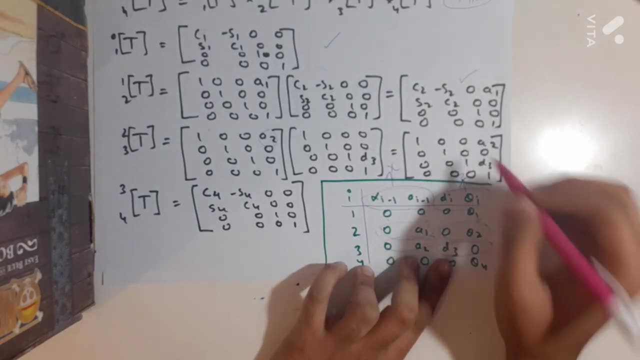 this is our translation a2 and this is our translation a2 and this is our translation a2 and this is our translation b3. so we multiply both of those to get this is along x and this is along z to get our final transformation matrix for 2 to 3, our 3 to 4. you can see there is nothing. 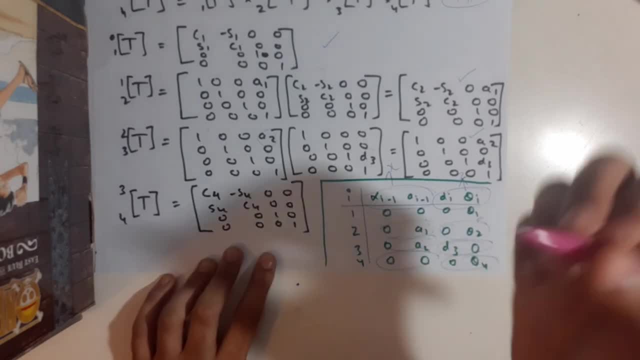 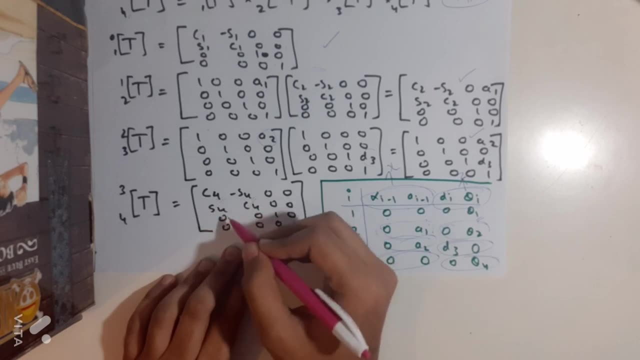 happening in our x axis. we are only rotating in the z axis. as you can remember, the last was the end effector and the end effector just rotates. so again we have theta 4. we are just going to rotate it by theta 4. so, as you can see, we have that transformation matrix set. now how do we obtain? 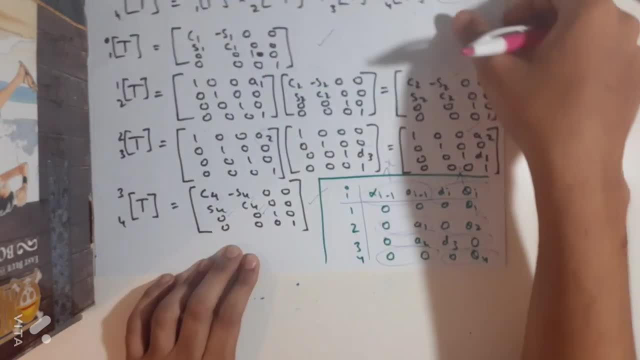 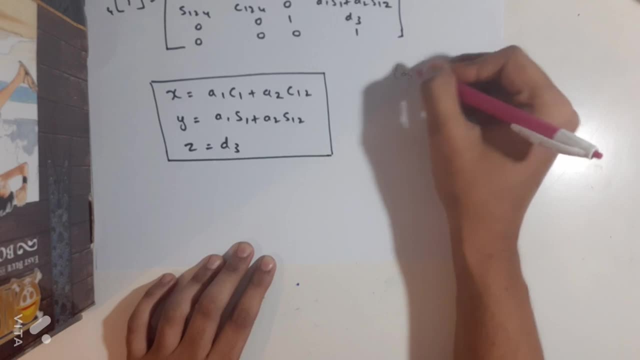 the final transformation matrix. we just rotate it by theta 4 and we have the transformation matrix set. multiply all of these together. so here we have done that. so what does 1 to 4 mean? basically, it means cos theta 1 plus theta 2 plus theta 4, like cos theta 1 plus theta 2 plus theta 4. this is just. 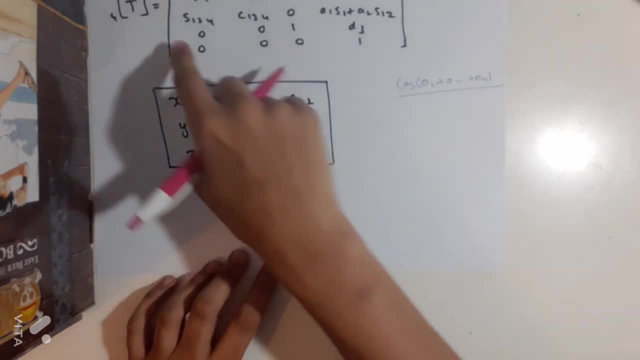 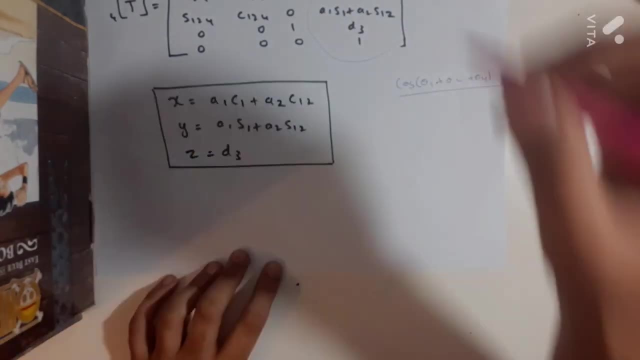 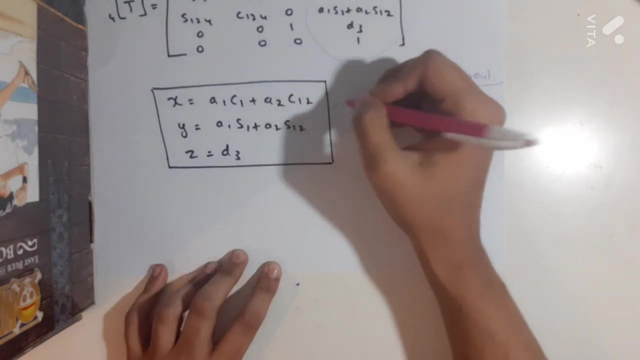 like a common notation. most of you must be aware of this. so we write that multiplication, totally. what we are actually interested in is this row, now, sorry, this column. what this is going to provide us with is it's going to provide us with x, y, z matrix. 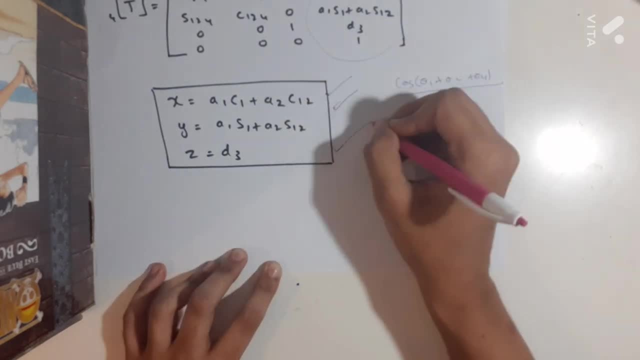 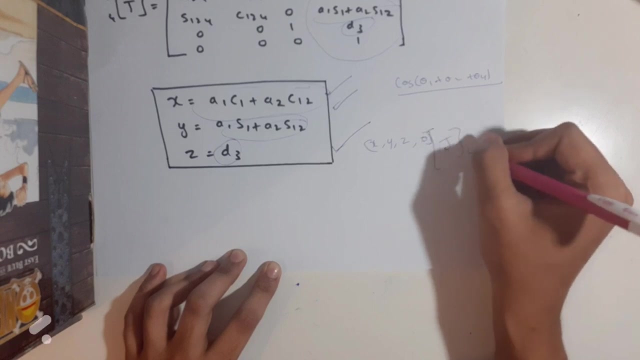 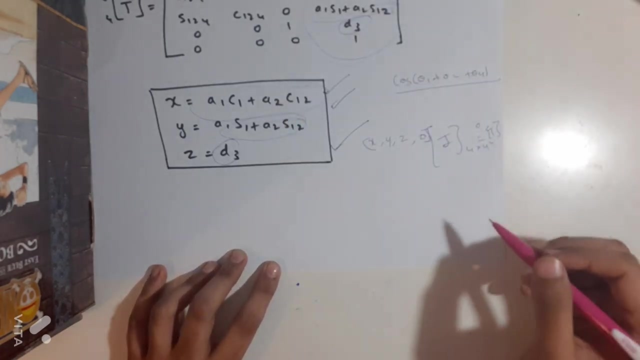 so x, y, z values which we were after. so this element is x, this is y and this is your z. you can think of it as x, y, z, 0 into like a identity matrix of 4 by 4 is equal to your transformation matrix 4, 0. so like you get these values in right now with our x, y z, we are going to get 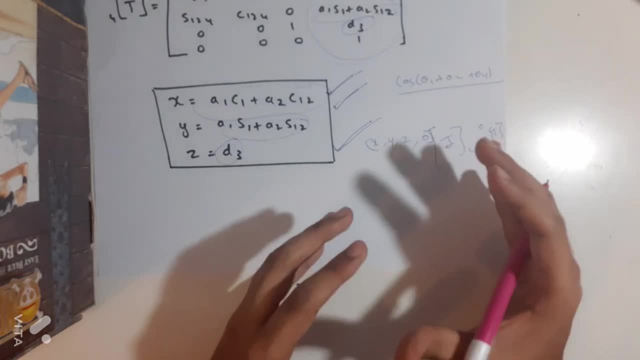 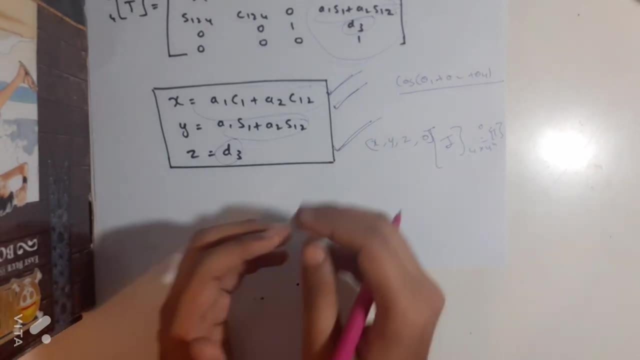 the x and y, z. here we are going to get the x- 0, and if you think about x, 1 of the x in the x is going to be x4 and 2, and then, if you think about it in the blank space, we have these values. it basically means that the teeth of the circulation is going to match. 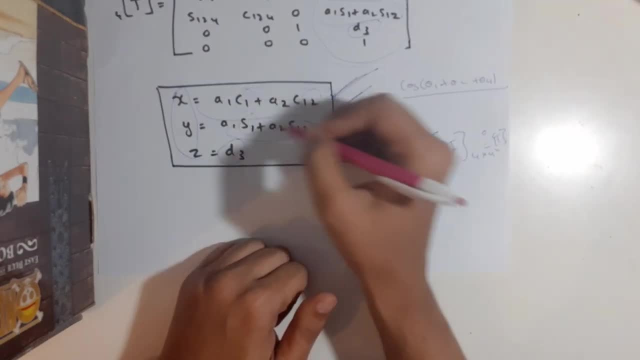 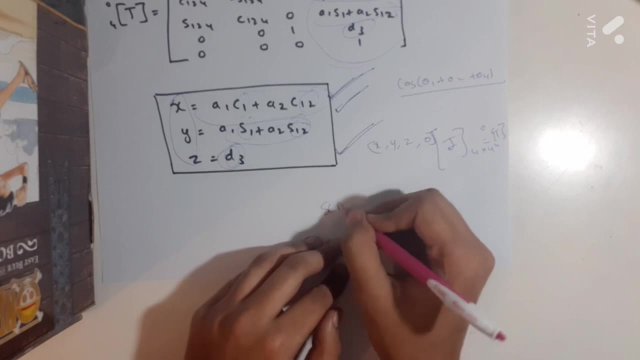 up to this problem and that for this situation, she is going to generalize, and then what she did is she is going to insert these values into the automatic derivative that she has here. so, for instance, right before i do so, let us essentially just use square and divide. 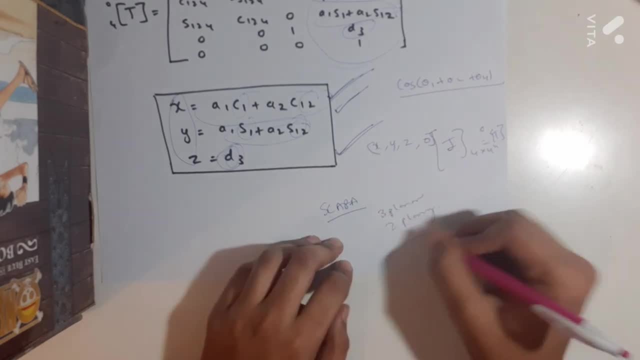 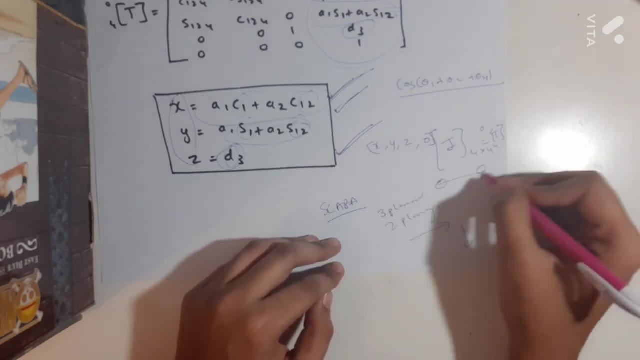